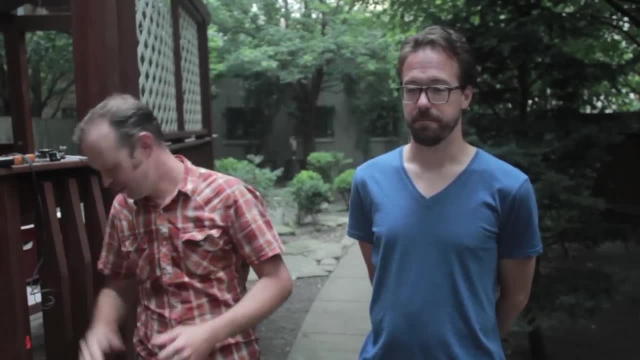 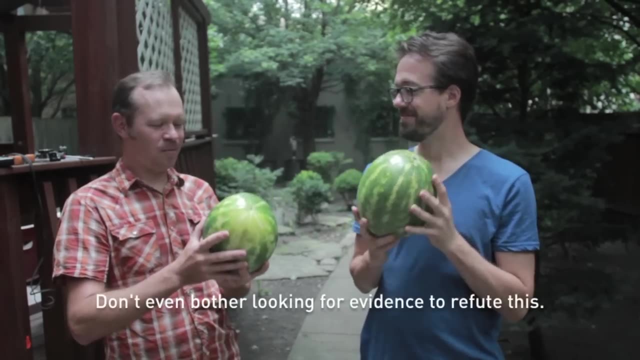 We're going to do some rigorous scientific experiments and we'll be back All right. so we've got our melons. Two human heads, Two human heads. We went and did a lot of research and found that some of these watermelons- 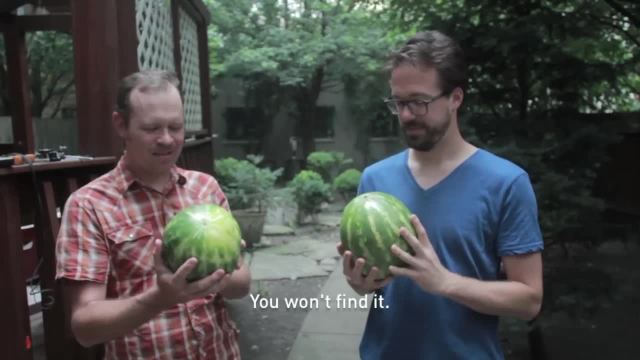 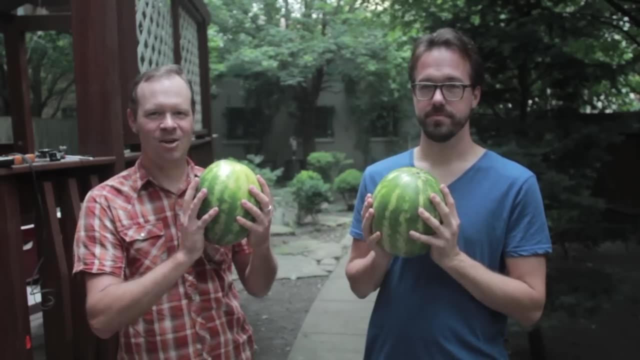 are actually identical to the human head in every respect: Weight, hardness, density. When you shake it around, you can hear the liquid inside. So yes, this is science, Respect it. okay, It's hard science. I've got this old helmet. 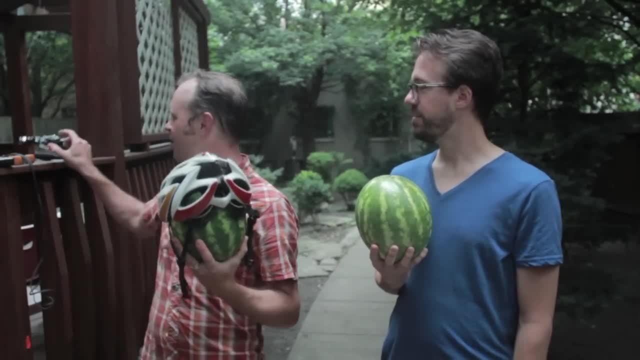 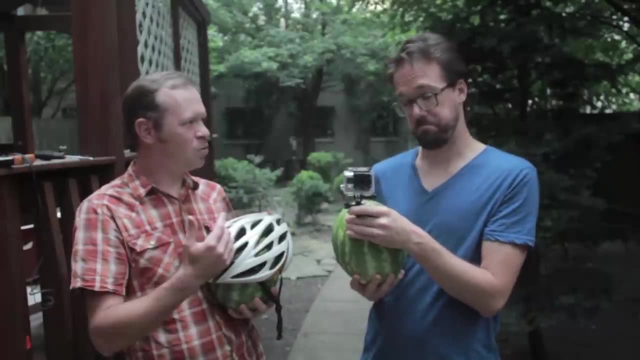 Found one that fits Jeff, has been kind enough to loan us his. This is the GoPro Hero 3, and you can take, I want to say, 200 frames per second, Which would let it slow it down to 10 times normal speed. 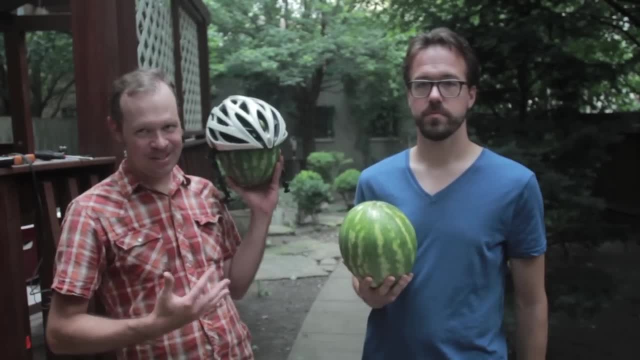 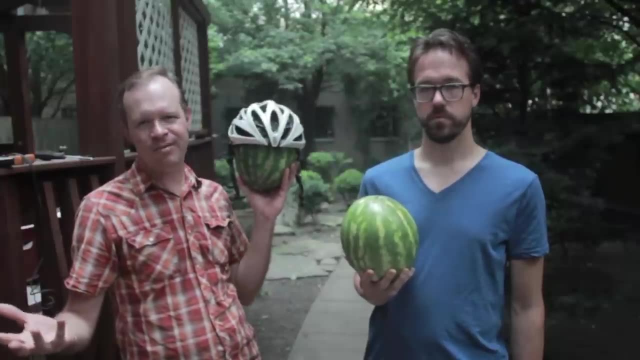 Super slow-mo is what you're going to see. We're going to try smashing the helmeted melon first, and hopefully we're going to see the helmet take the brunt of the force And then, maybe just Just for fun, we'll see what happens without a helmet. 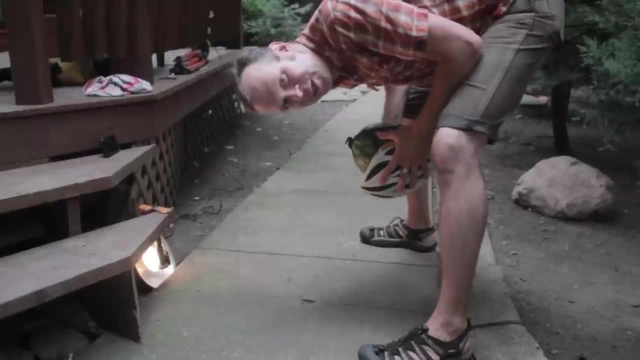 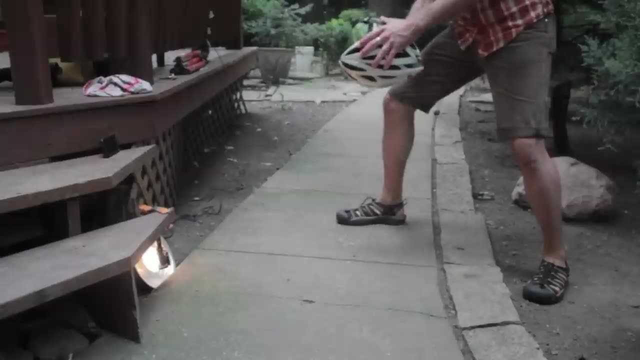 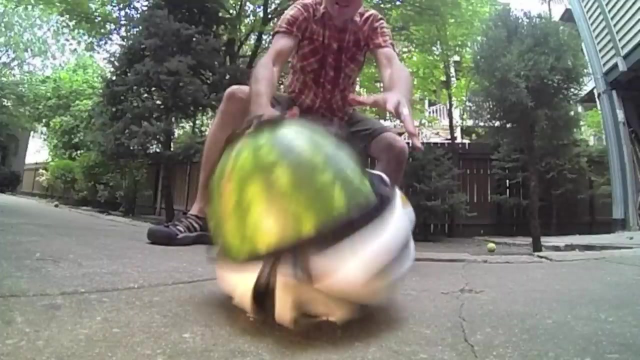 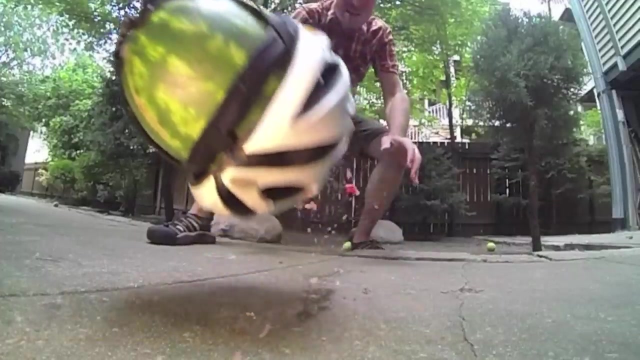 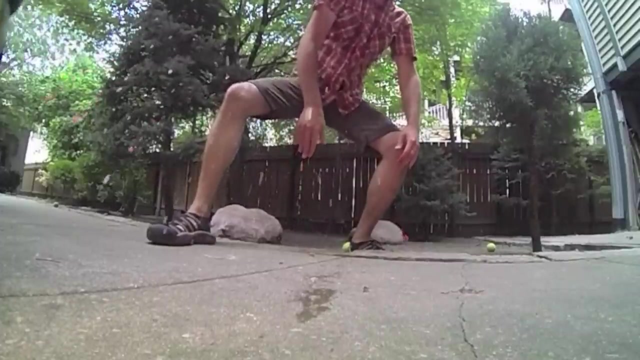 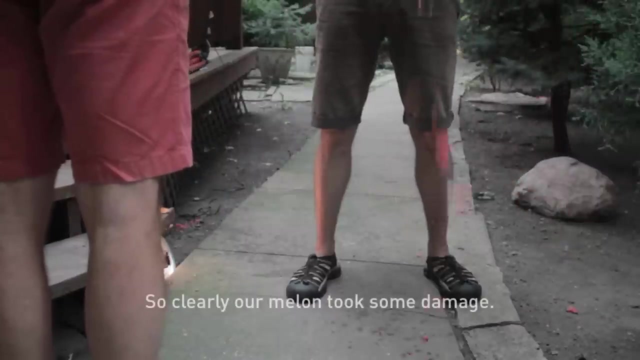 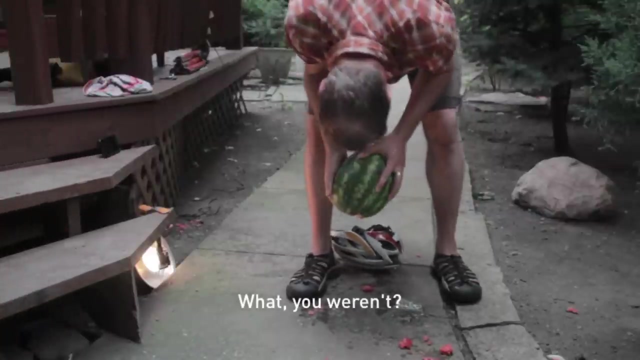 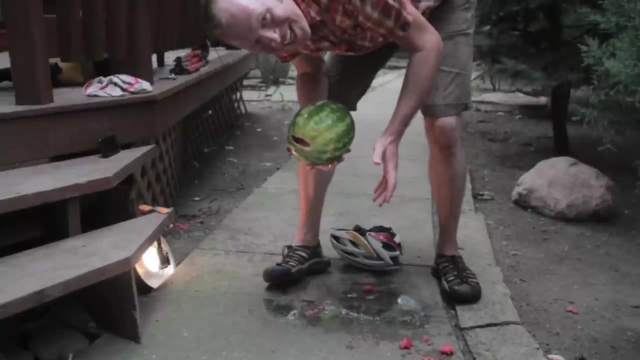 Yeah, All right. All right, let's do this. We're just going to do this, All right, All right, Fun. Well, there you have it, folks, But just as a compare and contrast, let's go ahead and try it. you want to try it once? 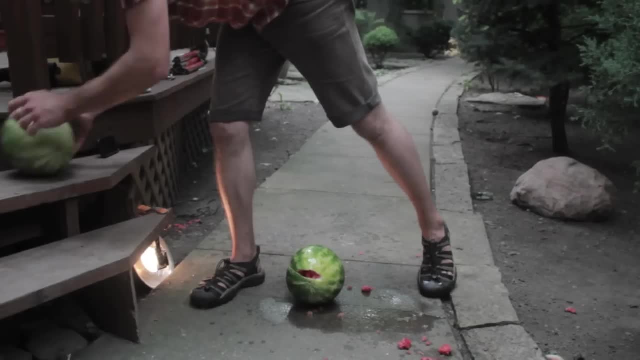 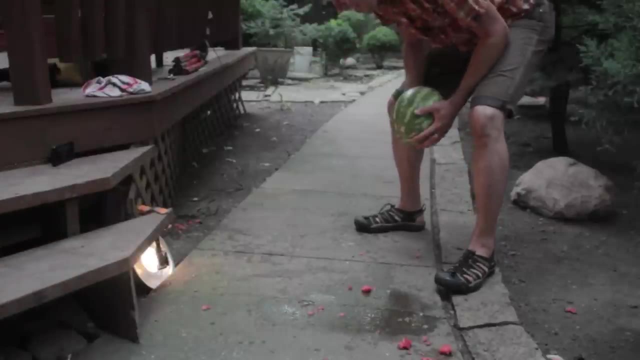 without a helmet? Yeah, All right, let's see what happens without the helmet. That thing's waterproof, right? Yeah, Okay, Totally waterproof. All right, here we go. Mmm, All right, here we go. All right, here we go. 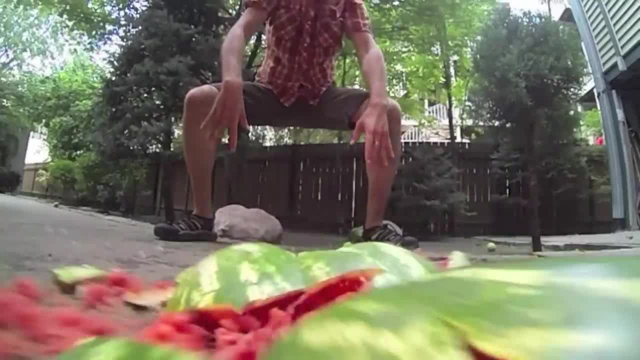 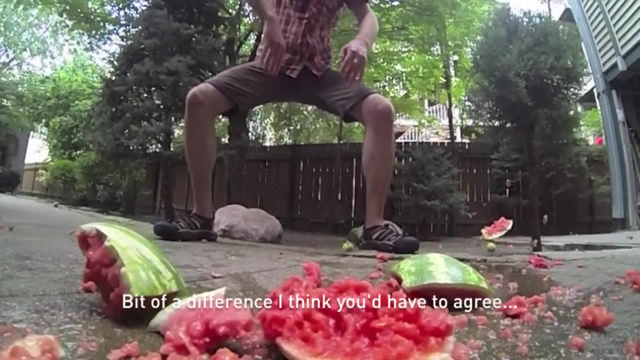